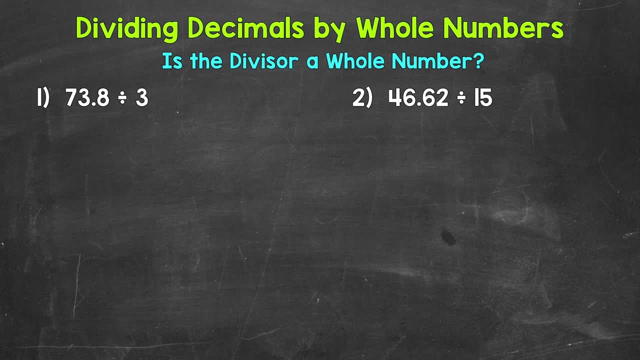 We'll start with dividing decimals by whole numbers and we will go from there. Now, decimals and division show up all throughout math and really throughout life as well. So being able to work with decimals and solve division problems involving decimals will be beneficial, no matter what class, level of math or goal you are working towards. 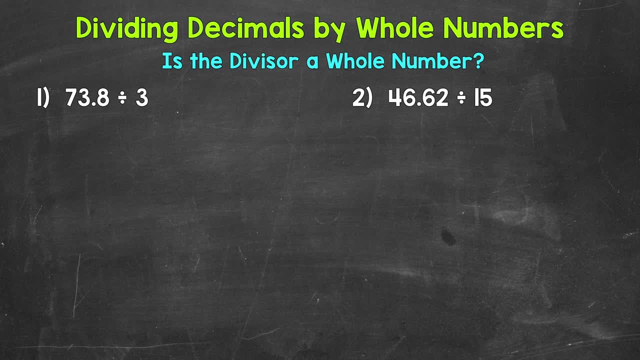 Whatever your situation may be, this should be helpful in better understanding how to divide decimals. Let's jump into number one, where we have 73 and 8 tenths divided by 3.. The first thing that we need to do is set this problem up. 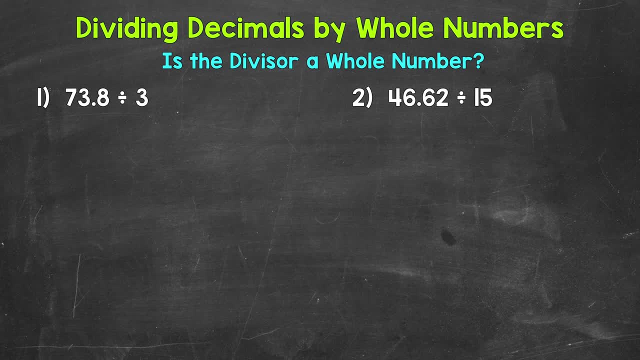 That way we can go through the division process. 73 and 8 tenths is the dividend, the number we are dividing, So it goes under the division bar. 73 and 8 tenths divided by 3.. 3 is the divisor, the number we are dividing by. 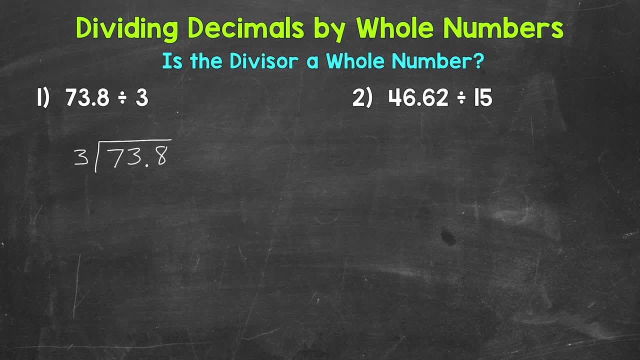 So it goes under and outside of the division bar. Now, whenever we have a division problem that involves decimals, we always need to check: Is the divisor a whole number? If yes, bring the decimal straight up into the answer. So for number one, our divisor is 3.. 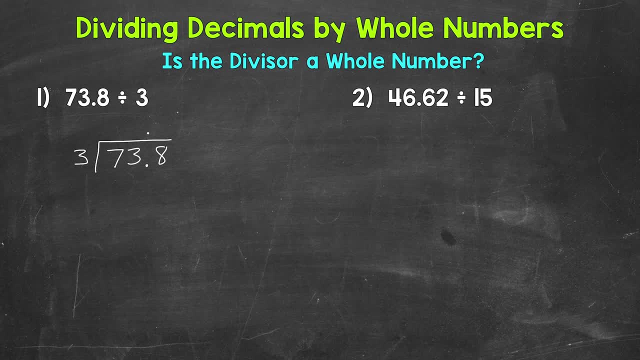 That's a whole number. So we bring the decimal straight up into the answer. Now we go through the division process, The same process we use when we divide by a number, whole numbers. So divide, multiply, subtract, bring down, repeat. We start with divide. So we have 7. 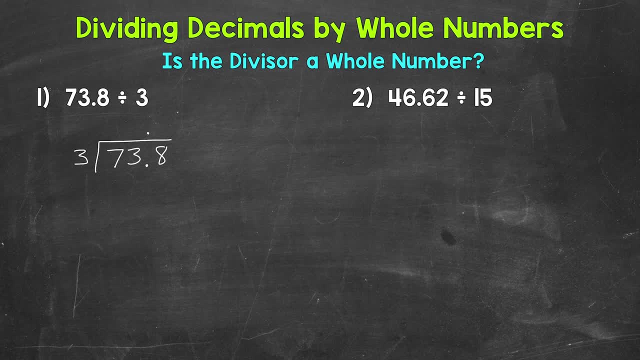 divided by 3. How many whole groups of 3 in 7? Well, 2.. That gets us to 6.. Now we multiply 2 times, 3 is 6.. Subtract 7 minus 6 is 1.. And then we bring down, Now we have 13, and we repeat, So we: 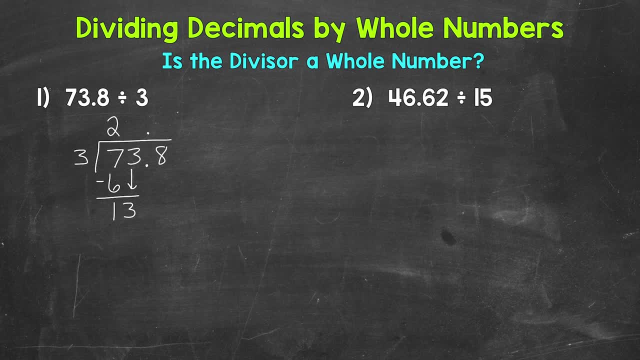 go back to divide. 13 divided by 3. How many whole groups of 3 in 13? 4. That gets us to 12.. Now we multiply 4 times 3 equals 12.. Subtract 13 minus 6 is 6.. Subtract 7 minus 6 is 1.. And then we bring. 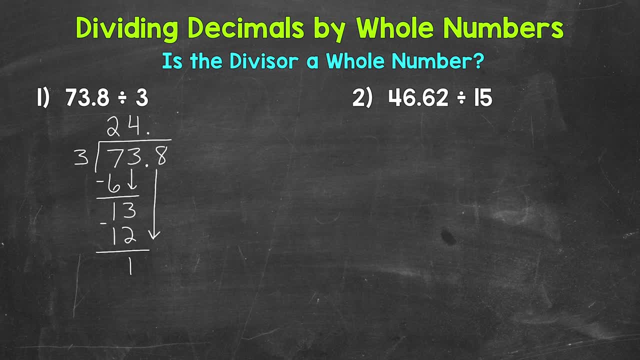 down The 8. Now we have 18 and we repeat. So we go back to divide 18 divided by 3.. So how many whole groups of 3 in 18? 6. That equals 18 exactly. Multiply 6 times 3. 18. Subtract And we get 0.. 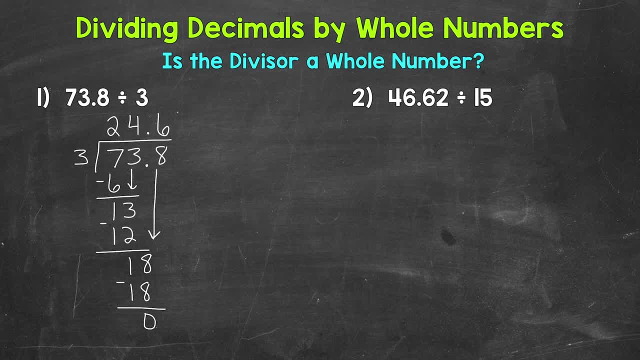 So we went all the way over to the further bottom. So we have 6.. Subtract And we get 0. So we went all the way over to the this place to the right, which was the tenths place for number 1. And we have a clean cut 0 here. 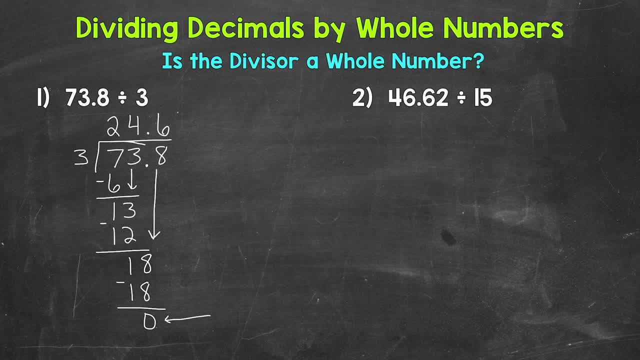 that tells us that we are done. Our final answer: 24 and 6 tenths For number 2, we will see what happens when we do not get that clean, cut 0 and we need to extend the problem until we do. 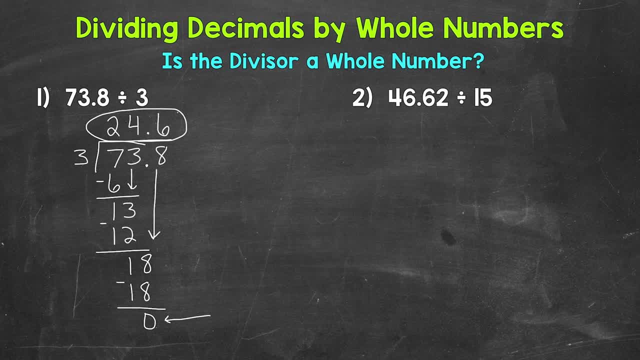 Let's move on to number 2, where we have 46 and 62 hundredths divided by 15.. Let's start by setting this problem up: 46 and 62 hundredths divided by 15.. Is the divisor a whole number? Yes, 15 is a whole number. That means we bring the decimal straight up into the answer. 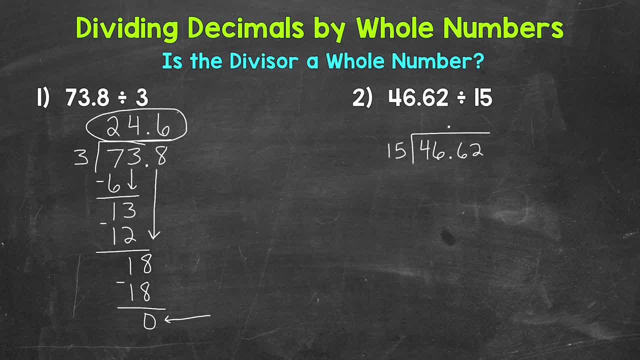 And now we go through the division process. So we start with divide. We have 4 divided by 15.. How many whole groups of 15?? We have 4 divided by 15.. How many whole groups of 15?? We have 4 divided. 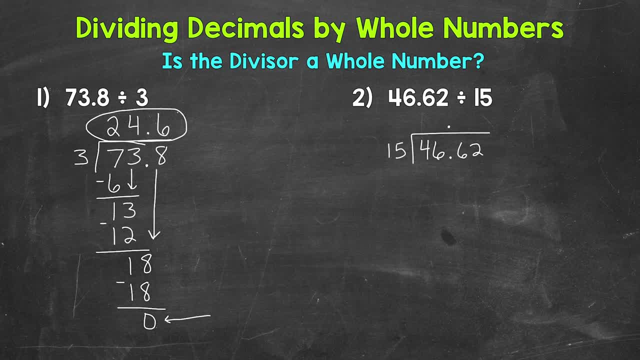 by 15 and 4.. Well, we can't do that, So we need to use the 6 as well and take a look at 46.. We have 46 divided by 15. How many whole groups of 15 in 46?? Well, 3.. That gets us to 45.. 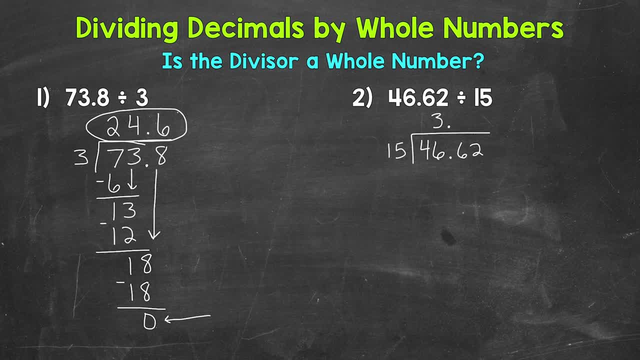 Make sure that 3 goes above the 6 in 46, not above the 4. Since we used both of those digits and we had 46 divided by 15, that 3 needs to go above the 6.. Now we multiply 3 times 15 is 45. Subtract 46 minus 45 is 1. And then bring down. 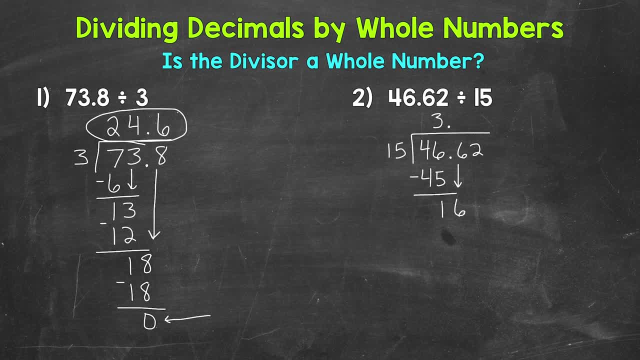 Now we have 16 and we repeat. So back to divide. 16 divided by 15.. How many whole groups of 15 in 16?? 1. Now we multiply 1 times 15 is 15.. Subtract 16 minus 15 is 1.. Bring down the 2. And now we have 12. So repeat and we go back to divide. 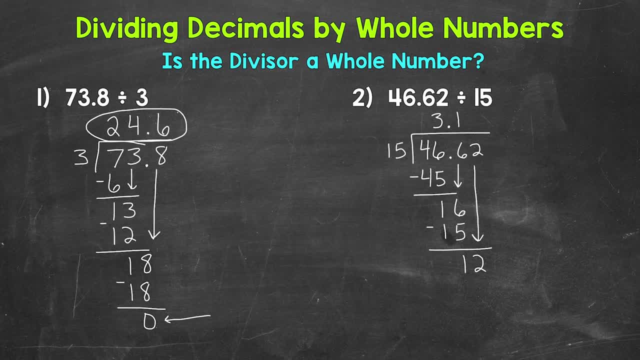 12 divided by 15.. How many whole groups of 15 in 12?? Well, we can't do that, So we need a 0 here And now. we multiply 0 times 15 is 0.. Subtract 12 minus 0 is 1.. And then we have. 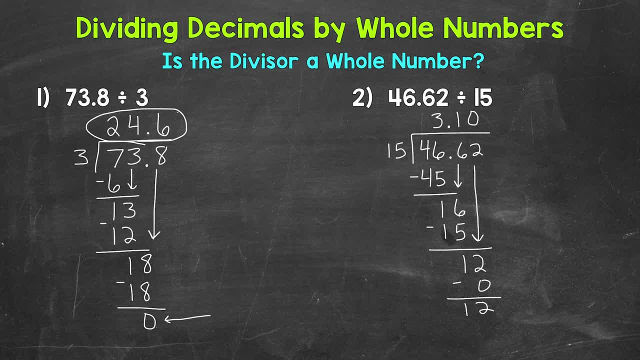 12.. So we went all the way over to the furthest place, to the right, the hundredths place, but we have a 12 at the end. We do not have a clean cut zero. yet That 12 does not mean remainder 12 like. 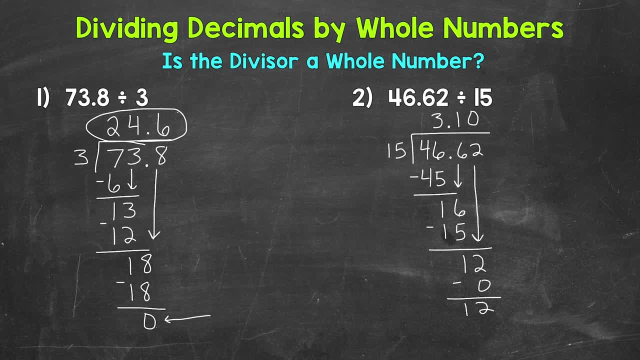 when we work with whole numbers. This answer is in decimal form, so we need to keep it that way. What we need to do is extend the problem until we do get a clean, cut zero, and that will mean the problem is done and we have our final answer. We can do this by using placeholder zeros that we 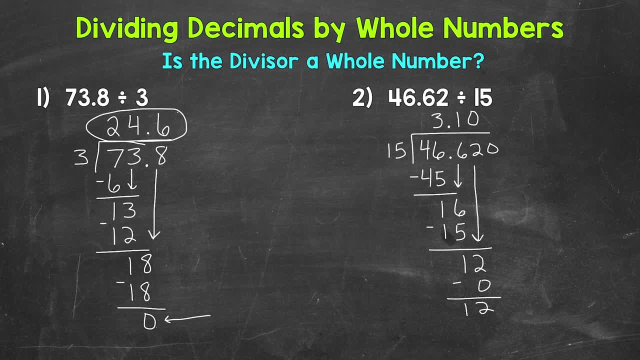 can bring down. So let's use a placeholder zero in the thousandths place that we can bring down and continue this problem in order to work towards that final answer. Now remember: zeros to the right of a decimal do not change the value of that decimal, of that number, so we are able to use 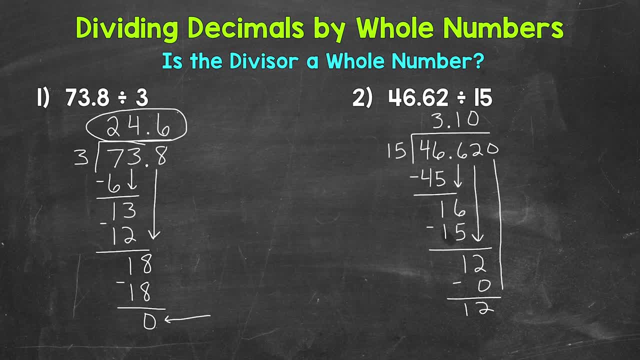 this strategy. Let's bring this zero down and continue the problem. So now we have 120 and we repeat. so we go back to divide. We have 120 divided by 15.. How many whole groups of 15 in 120?? Well, 8, and that hits. 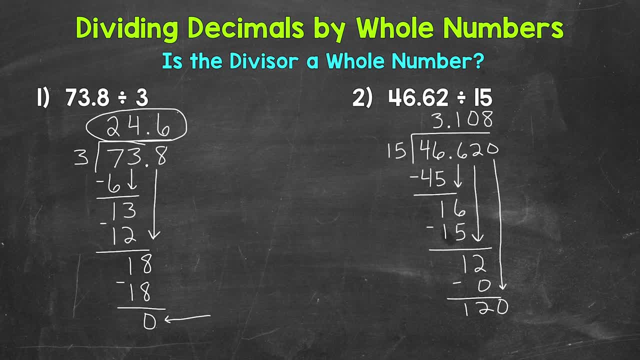 120. exactly Now, we multiply 8 times 15 is 120.. Subtract 120 minus 120. Subtract 150 plus 120 is 0.. So now we have that clean cut zero and we are done with this problem. We have our final answer: 3 and 108 thousandths. So there's how we divide decimals by whole numbers. 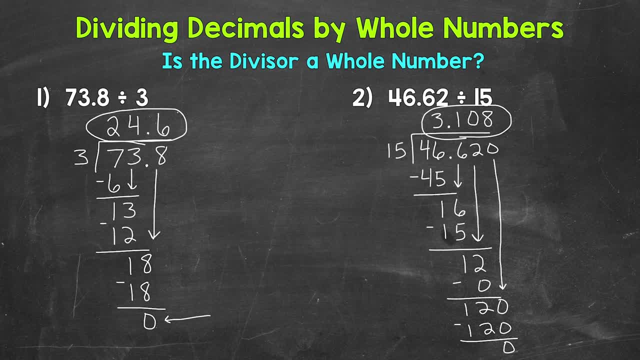 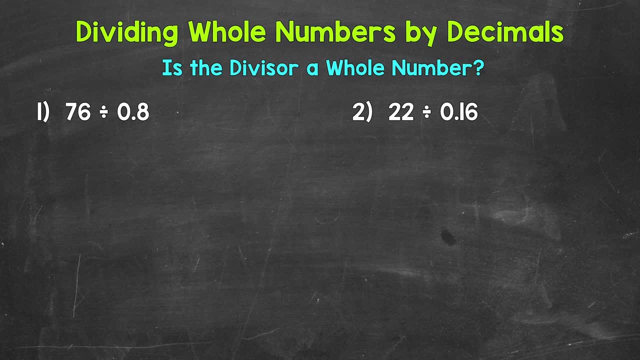 Let's move on to dividing whole numbers by decimals. Here are our examples of dividing whole numbers by decimals. Let's jump into number one, where we have 76, divided by 8 tenths. The first thing that we need to do is set this problem up. That way we can go. 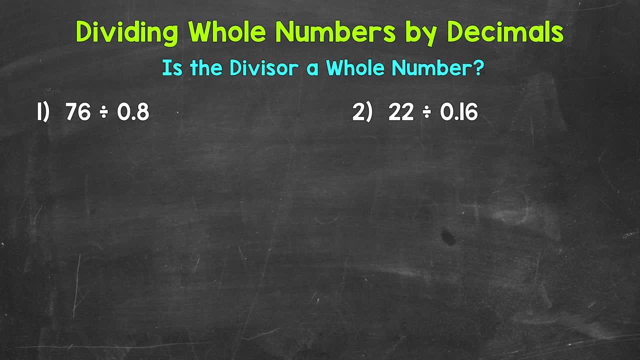 through the division process. 76 is the dividend, the number we are dividing. It goes under the division bar. 8 tenths is the divisor, the number we are dividing by It goes on the outside of the division bar. Now, whenever we have a division problem that involves decimals, we always need 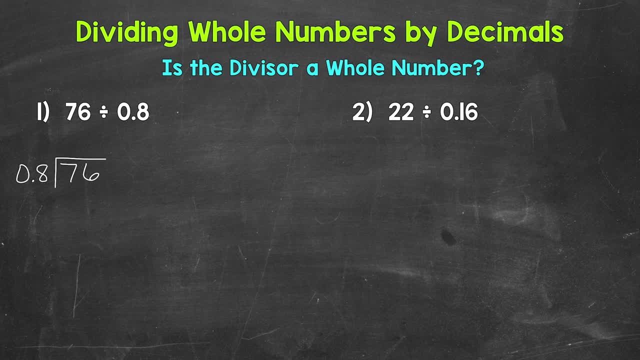 to check: Is the divisor a whole number? Our divisor for number one is 8 tenths. 8 tenths is not a whole number. That means we need to make it a whole number. Let's move the decimal once to the right to make that a whole 8.. Now, technically speaking, we need to multiply the divisor by a. 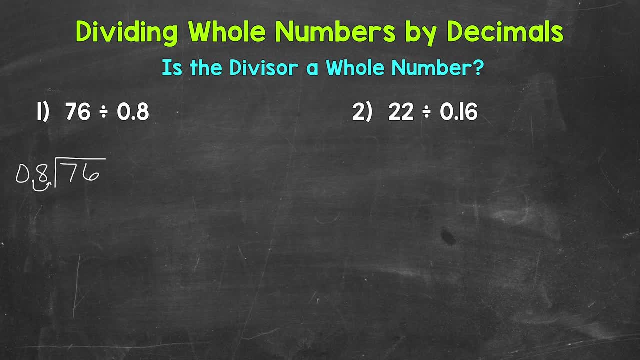 power of 10 in order to make it a whole number, For example number one, we multiplied 8 tenths by 10.. That shifted the digits one place to the left, therefore giving us a whole 8.. But we made that. 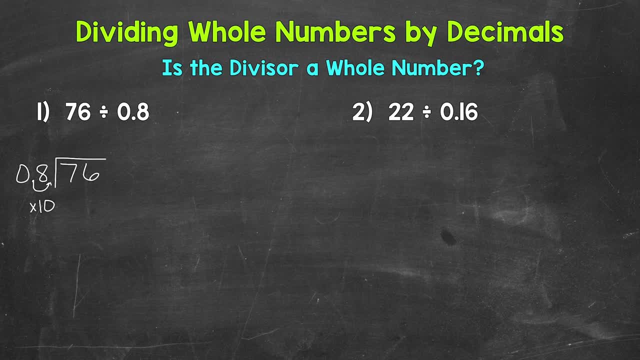 process a little simpler to think through by just thinking of this as moving the decimal to make the divisor whole. Now, whatever we do to the outside, the divisor, we must do to the inside, the dividend. So if we multiply the outside by 10, we need to multiply the inside by 10 as well. 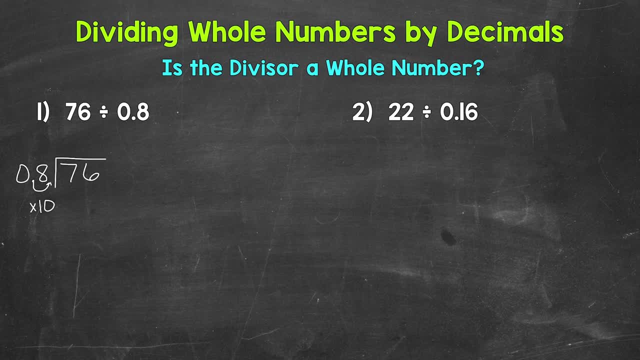 to keep this problem balanced. So let's move the decimal once to the right on the inside. Now 76 is a whole number, so the decimal comes after 76 and any other whole number. Let's move it once to the right. fill this with a 0, and we multiplied our dividend by 10 as well. Now that we have 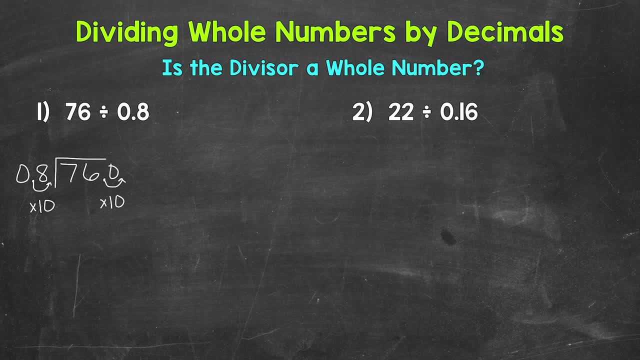 our whole divisor. let's rewrite this equivalent problem to the side. So we have 760 divided by 8.. Now our divisor is whole, so we can go through the division process. So divide, multiply, subtract, bring down, repeat. Let's start with divide. So we have 7 divided by 8.. 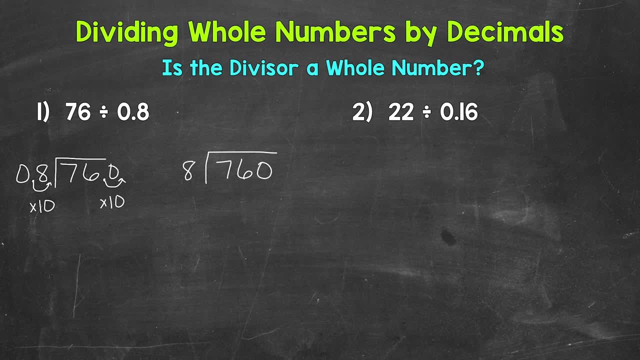 How many whole groups of 8 in 7?? Well, we can't do that, So we need to use the 6 and take a look at 76.. 76 divided by 8.. How many whole groups of 8 in 7?? Well, we can't do that, So we need to use 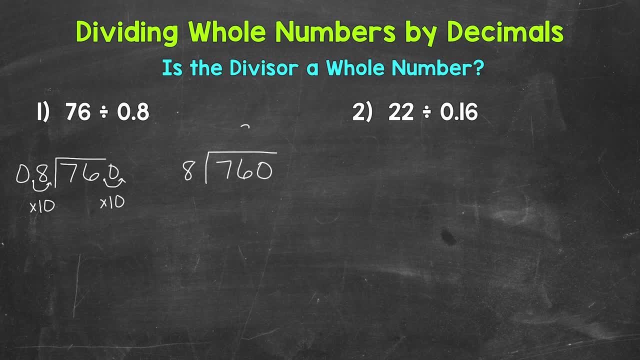 the whole groups of 8 in 76. 9.. That gets us to 72., And that 9 needs to go above the 6, not above the 7, because we used 76 there. Now we multiply 9 times 8, 72.. Subtract 76 minus 72: 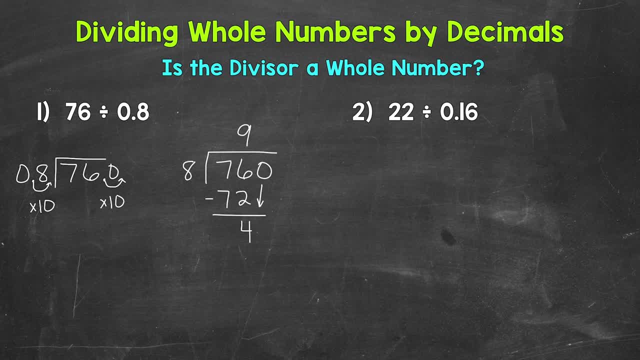 gives us 4. Then we bring down And then repeat. So we go back to divide. Now we have 40 divided by 8. How many whole groups of 8 in 40?? Well, 5.. That gets us to 40. 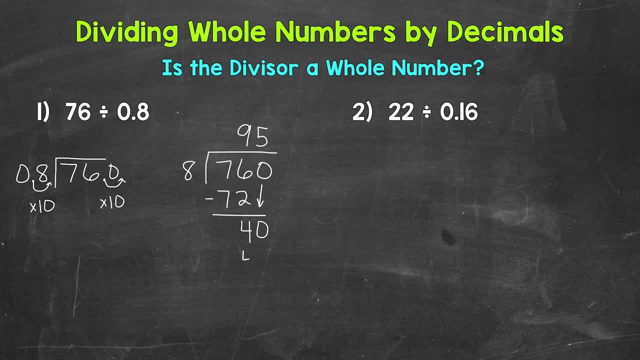 exactly: Multiply 5 times 8, 40.. Subtract 40 minus 40 is 0.. We went all the way over to the furthest place to the right. We have a clean cut 0 at the end here. So we are done, Our final answer. 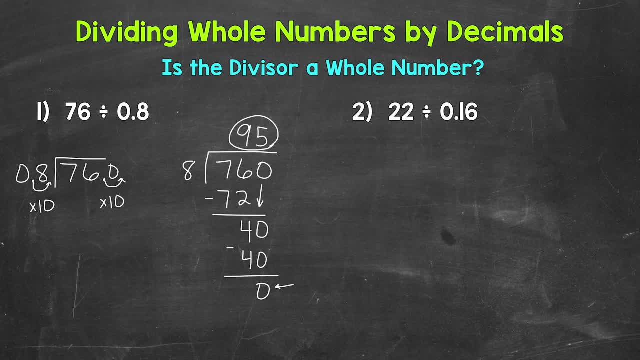 95.. Now for number 1, we have a whole number answer. We went all the way over to the furthest place to the right in our dividend as far as bringing digits down And we have a clean cut 0 at the end. So we do not have a decimal part of our answer Again, we have a whole number answer. 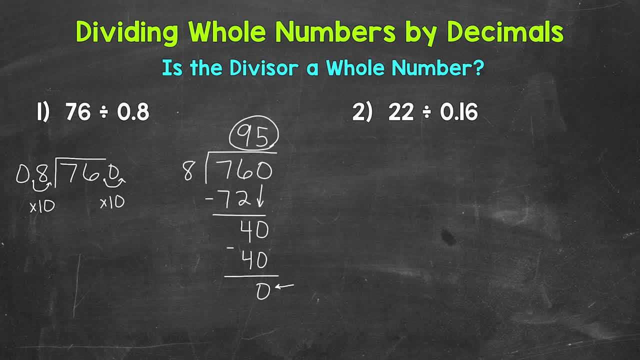 In number 2, we will see what happens when we do have a decimal part of our answer. Let's move on to number 2, where we have 22 divided by 16 hundredths. Let's set this problem up So we have 22.. That's our dividend, the number we are dividing. 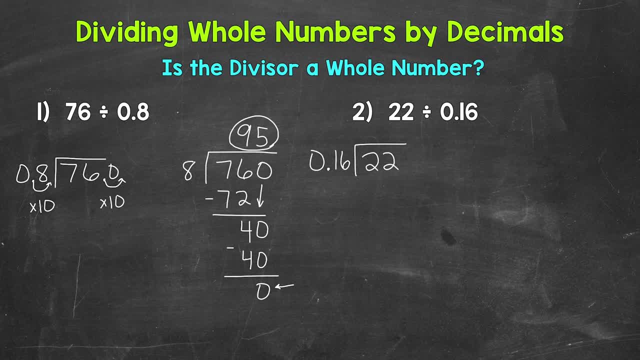 And then 16 hundredths is our divisor, the number we are dividing by. Is the divisor a whole number? 16 hundredths is not a whole number, So let's make it a whole number by moving this decimal twice to the right, And that's going to be a whole 16. now, 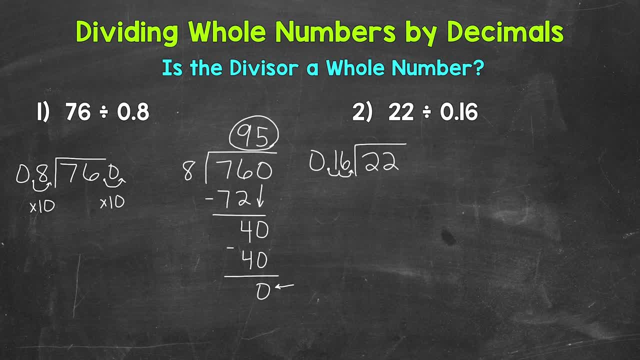 Now, technically, We shifted the digits of 16 hundredths two places to the left to make that a whole 16.. The power of 10 that we multiplied by was 100. Now, since we multiplied the divisor by 100, we need to multiply the dividend by 100. 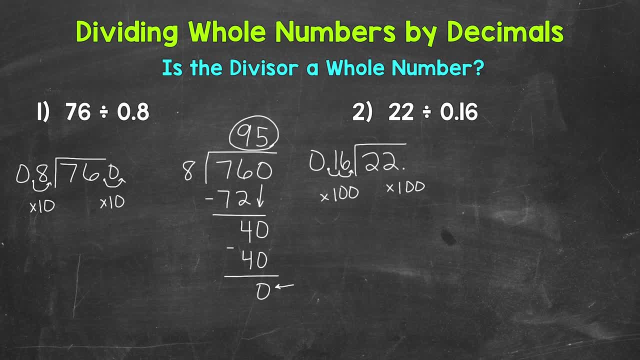 Let's move that decimal twice, so the decimal comes after 22.. Once twice, fill those gaps with zeros and we have our equivalent problem that we can rewrite and solve. So we have 2,200 for our dividend divided by 16.. 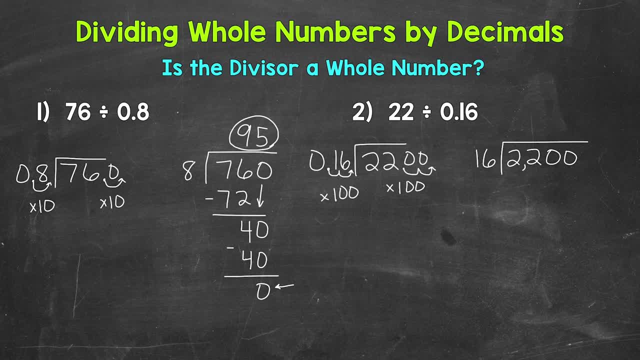 So now our divisor is whole and we can go through our process. Start with divide, So we have two divisors. How many whole groups of 16 in 2?? Well, we can't do that, so we need to use 22.. 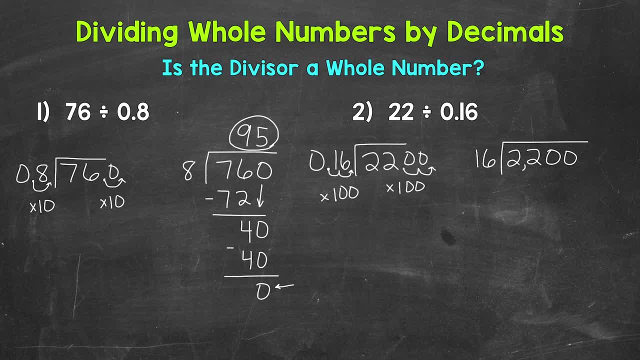 22 divided by 16. How many whole groups of 16 in 22?? 1. That 1 needs to go above the 22,. not that first 2,, since we used both of those digits and took a look at 22.. 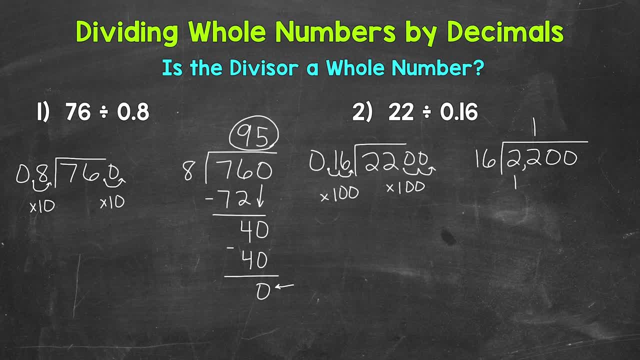 Now we multiply 1 times 16 is 16.. Subtract: 22 minus 16.. Let's borrow: It's a 1 there, and we have 12 minus 6, which is 6, and then 1 minus 1 is 0.. 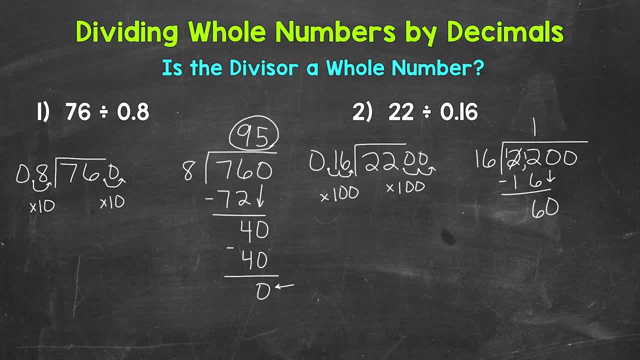 Now we can bring down this 0, and we have 60.. So we need to repeat and we go back to divide: 60 divided by 16.. How many whole groups of 16 in 60?? Well, 16 times 3 is 48.. 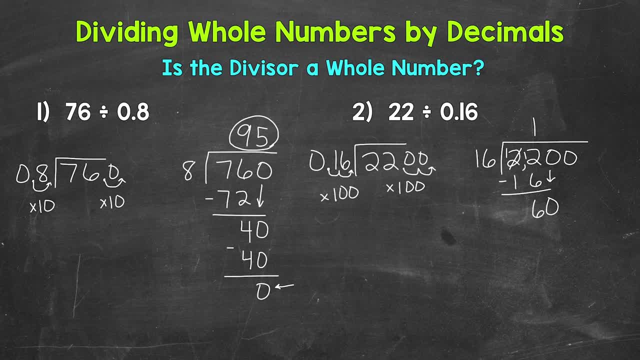 16 times 4 is 64.. 4 is too many, It's going to be 3.. Multiply 3 times 16.. 48. Now we subtract So 60 minus 48.. 0 minus 8.. 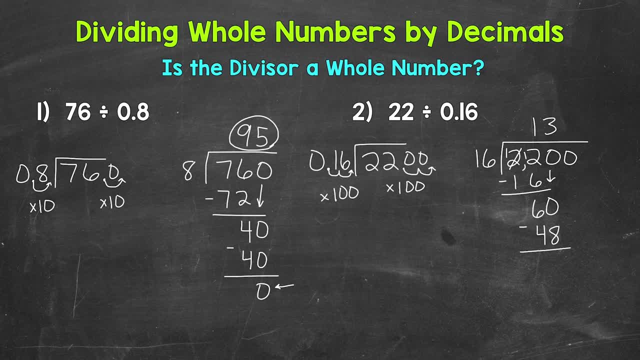 Well, we need to borrow here: 10 minus 8 is 2, and then 5 minus 4 is 1.. So 60 minus 48 equals 12.. Let's bring down that next 0.. Now we repeat: 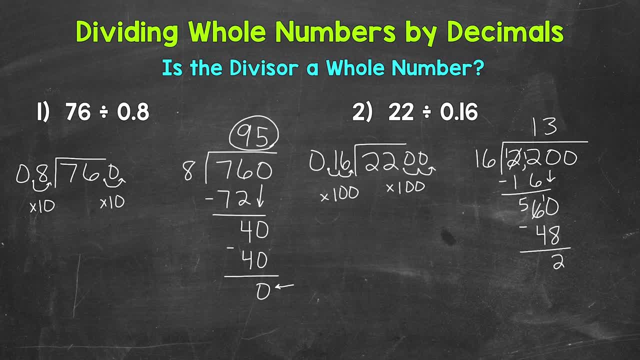 So we go back to divide: We have 1., We have 2.. We have 3.. We have 6.. We have 4.. We have 5.. We have 6.. We have 4.. We have 6.. 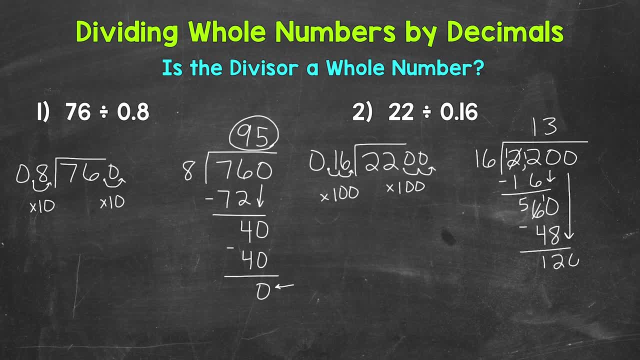 We have 5.. We have 5., We have 6., We have 6., We have 5., We have 6., We have 7., We have 7., We have 8.. We have 9.. We have 8.. 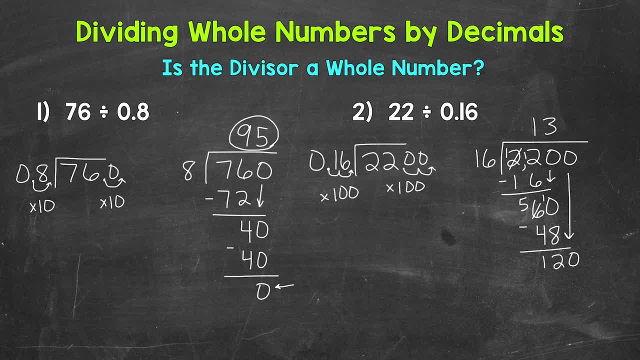 We have 9.. We have 10.. We have 11.. Okay, so we're going to find out how many whole groups of 16 are in 120.. How many whole groups of 16 in 120?? Now, you may not know how many whole groups of 16 are in 120 using mental math. 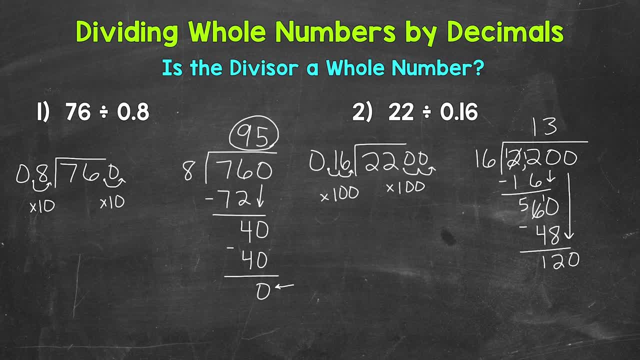 So we can estimate and check in order to find out. So I'm going to come to the side and use 16 times 10 as our reference point. So our starting point: 16 times 10 is 120.. is 160. That's kind of close to 120, so we can adjust based on that. Let's try 16 times 8. 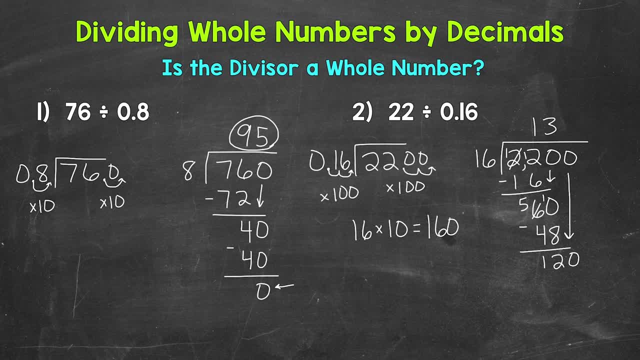 and see how close to 120 we get: 16 times 8.. So 8 times 6, 48.. 8 times 1 is 8, plus 4 is 12. 128. So 8 groups of 16, that's too many. Let's try 7.. 16 times 7.. 7 times 6, 42.. 7 times 1,. 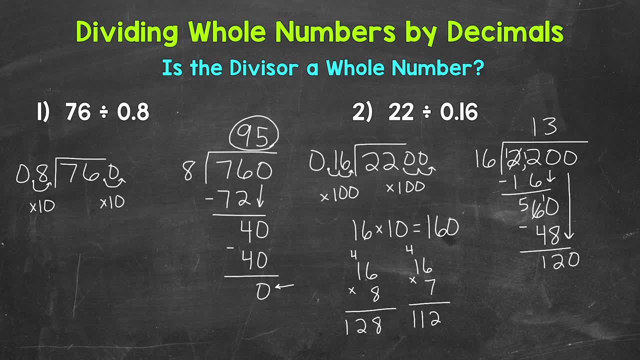 7 plus 4 is 11.. 112.. So it's going to be 7 groups of 16.. Let's put our 7 up here. Multiply 7 times 16, 112.. 112.. Subtract 120 minus 112.. Let's start with 0 minus 2.. We need to borrow. 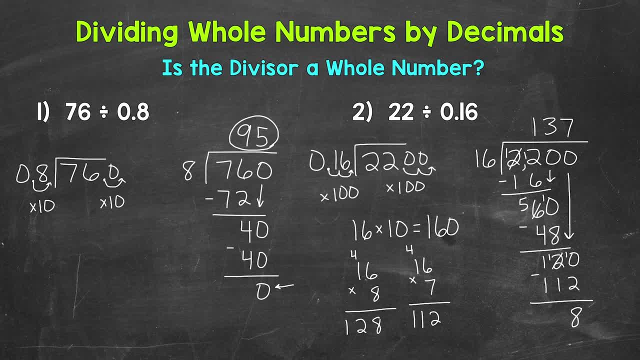 So that's 10 minus 2,, which is 8.. And then we have: 1 minus 1 is 0, and then another 1 minus 1, which is 0. So we end up with 8.. Now we went all the way over to the furthest place to the right. 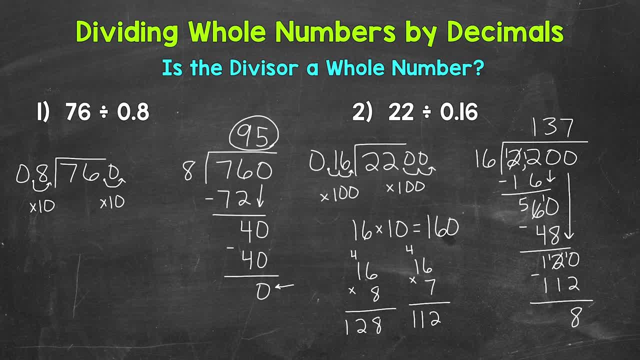 within our dividend so we do not have anything else to bring down. But we do not have a clean cut 0 at the end We have an 8.. We do not want to write 137 remainder 8.. We are working with decimals, So we want everything within our problem to be in decimal. 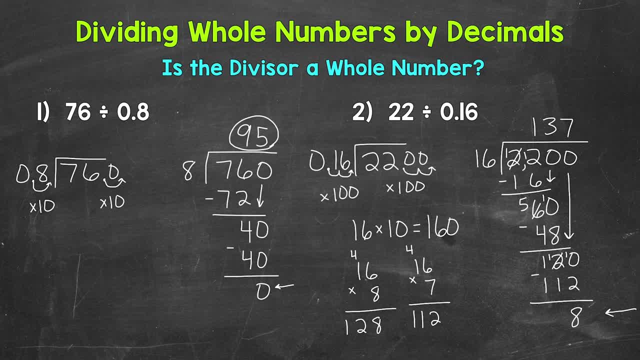 form, including our answer. So we need to continue this problem until we do get a clean cut 0.. So what we can do: we can include the decimal in our dividend and then bring it straight up into our our answer. Now we need something to bring down in order to continue this problem. So what we can. 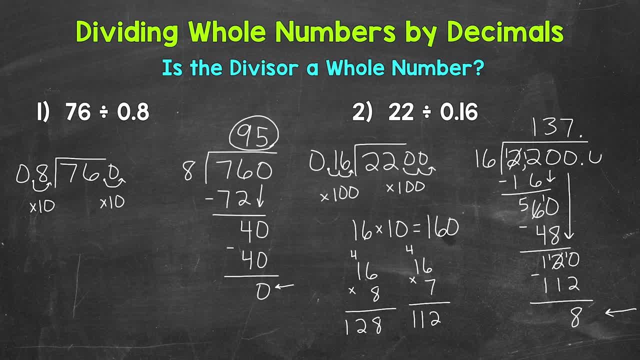 do? we can use placeholder 0s to bring down- Remember 0s to the right of a decimal or decimal digits do not change the value of that number. So we are able to use this strategy in order to continue the problem. Let's bring this 0 down and continue the problem. 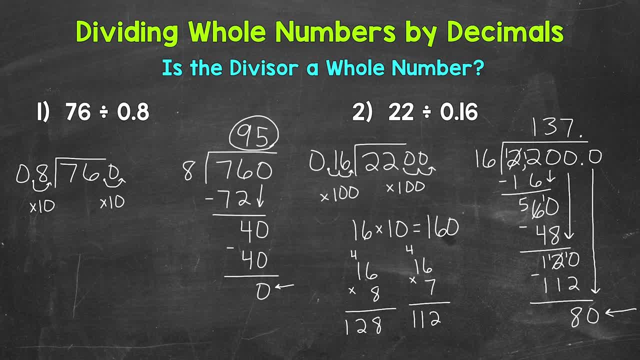 Now we have 80 and we can repeat. So we go back to divide 80 divided by 16.. How many whole groups of 16 in 80?? Well, 16 times 5 hits 80 exactly, So it's going to be 5.. 5 times 16 is 80.. 80 minus 80 is 0.. So we went all. 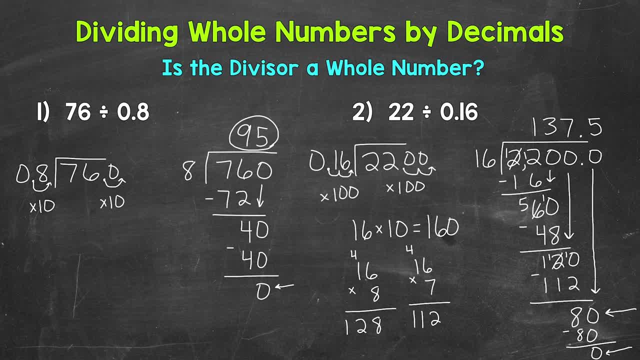 the way over to the right. Now we have that clean-cut zero. so we are done. Our final answer: 137 and 5 tenths. So there's how we divide whole numbers by decimals. Let's move on to dividing decimals by decimals. 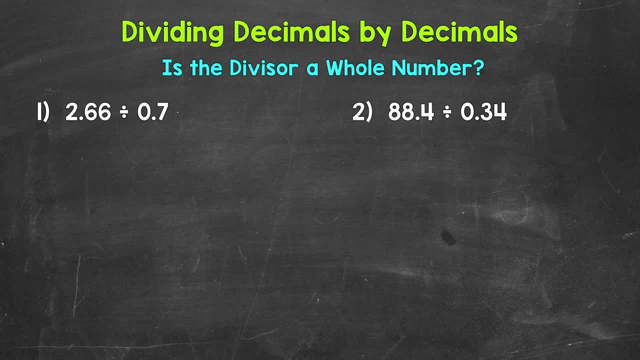 Here are our examples of dividing decimals by decimals. Let's jump into number 1, where we have 2 and 66 hundredths divided by 7 tenths. The first thing that we need to do is set this problem up. That way we can go through the division process. 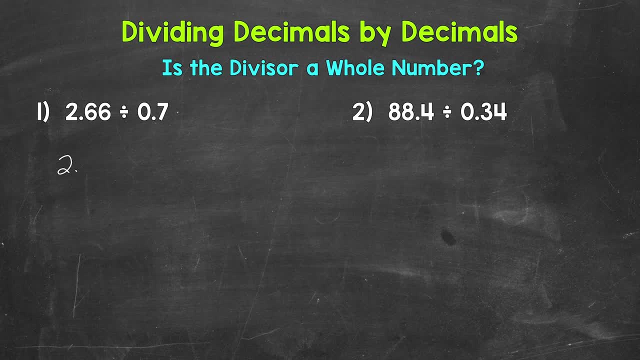 2 and 66 hundredths is the dividend, the number we are dividing. It goes under the division bar. 7 tenths is the divisor, the number we are dividing by. It goes on the outside of the division bar. Now, whenever we have a division problem that involves decimals, 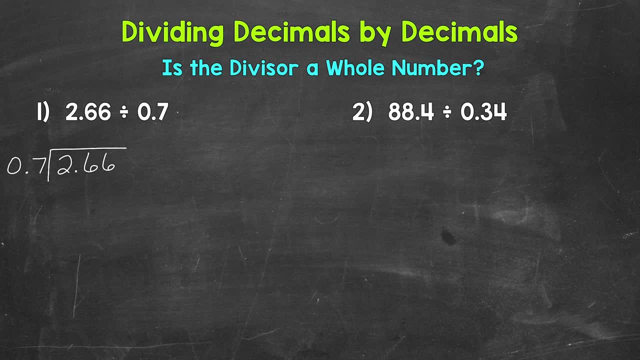 we always need to check: is the divisor a whole number? Well, 7 tenths is our divisor. That's not a whole number, So we need to make it a whole number. We can do this by moving the decimal once to the right. 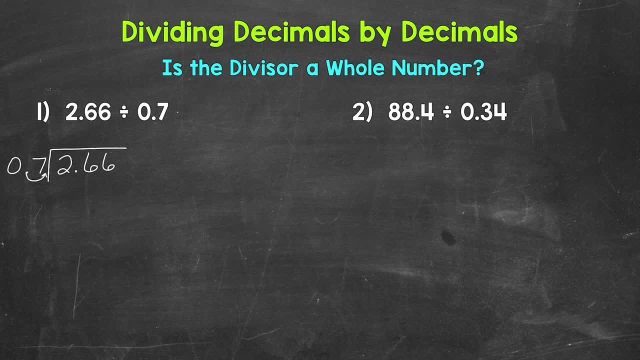 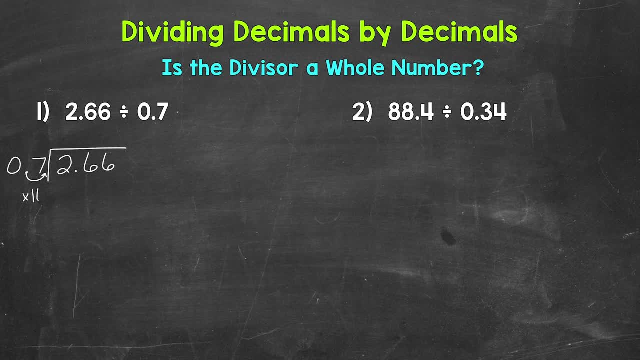 In the case of number 1, that power of 10 was 10.. So we multiplied 7 tenths by 10. This shifts the digits of our divisor to the left and gives us a whole number. We made this process simpler to think through by just thinking of this as moving the decimal. 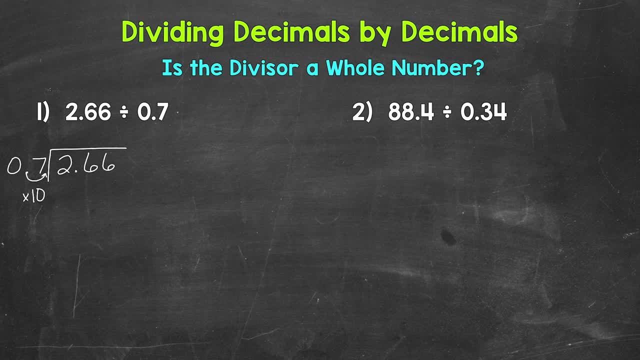 to make the divisor whole. Now, whatever we do to the outside the divisor, we must do to the inside, the dividend, in order to keep this problem balanced and equivalent. So we need to multiply the dividend by 10 as well. Let's move. 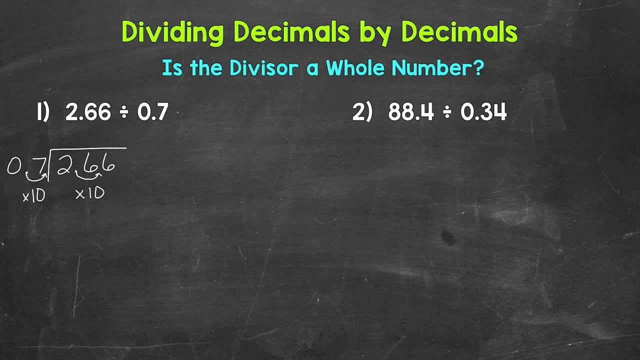 this decimal once to the right. Now we can rewrite our new equivalent problem with the whole divisor. So we have 26 and 6 tenths for our dividend and then 7 for our divisor. So is our divisor now a whole number? Yes, So we can bring our decimal straight up into our answer and now go. 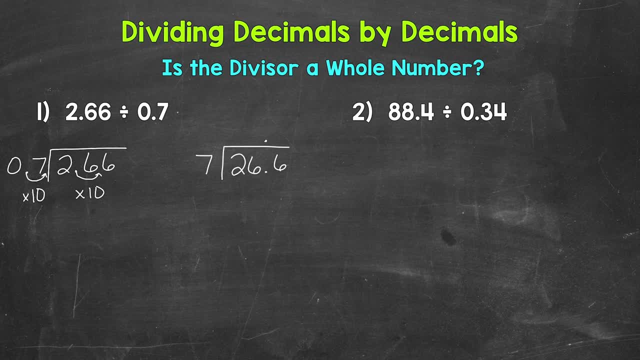 through the division process. So divide, multiply, subtract, bring down, repeat. Let's start with division: Divide. So we have 2 divided by 7. How many whole groups of 7 in 2?? Well, we can't do that. 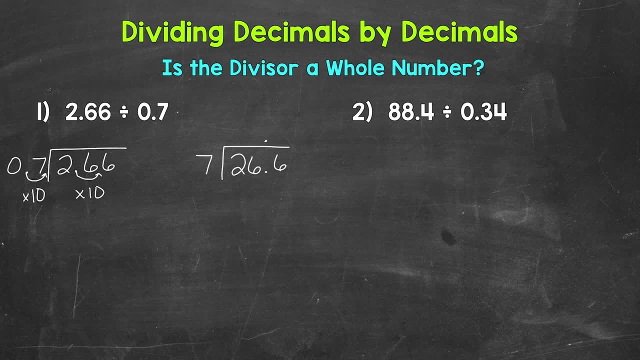 so we need to use the 6 and take a look at 26. We have 26 divided by 7. How many whole groups of 7 in 26?? Well, 3.. That gets us to 21.. Let's put the 3 above the 6 in 26,, not above the 2.. 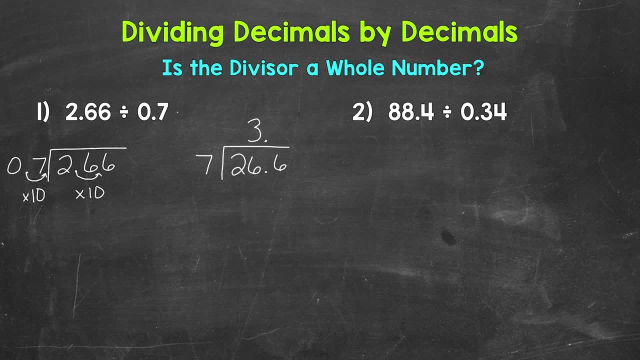 It needs to go above the 6, since we did 26 divided by 7.. Now we multiply 3 times, 7 is 21.. Subtract 26 minus 21 gives us 5.. Bring down Now we have 56 and we repeat. So we go back to divide. We have 56 divided by 7.. How many whole groups of 7? 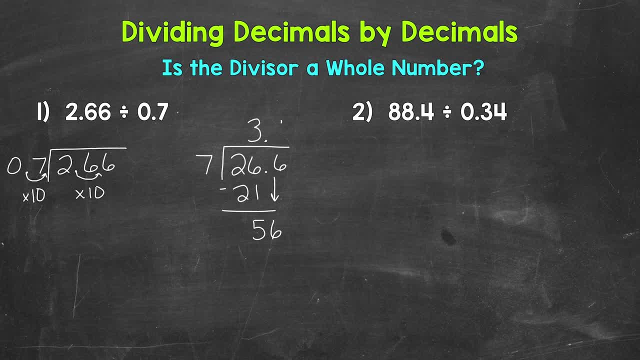 in 56?? Well, 8.. That hits 56. Exactly, Multiply 8 times 7.. 56.. Subtract 56 minus 56 is 0.. We went all the way over to the right within our dividend as far as bringing digits down, and we have a clean cut 0 at the end. So we are done. 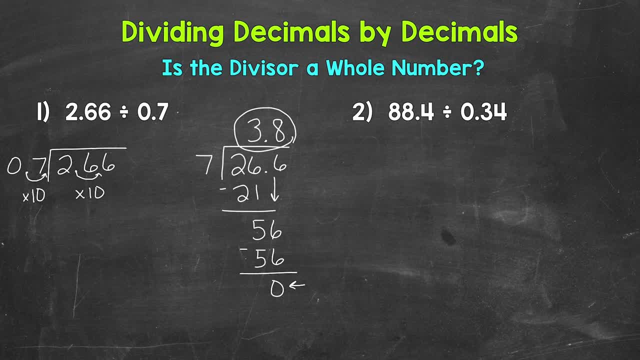 Our final answer: 3 and 8 tenths. Let's move on to number 2, where we have 88 and 4 tenths divided by 34 hundredths. Let's set this problem up: We have 88 and 4 tenths divided. 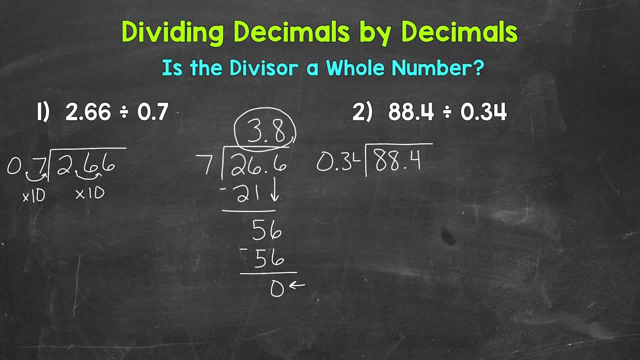 by 34 hundredths Is the divisor a whole number? No, 34 hundredths is not a whole number, So let's make it a whole number. Let's move the decimal once and then twice, So now we have a whole 34.. Now, technically, we multiplied that divisor by 100. That was the power of 10 that we 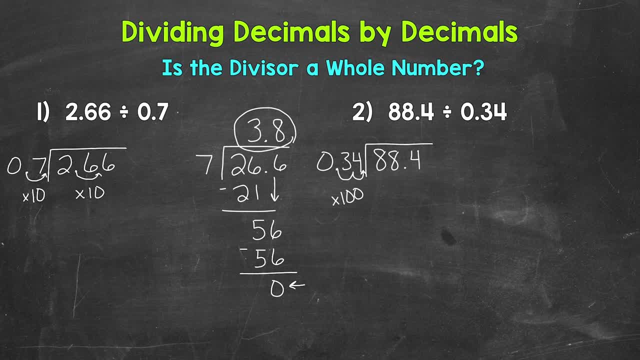 multiplied the divisor by, So those digits shifted two places to the left in order to give us a whole number. Now, whatever we do to the outside the divisor, we must do to the inside the dividend. So let's multiply 88 and 4 tenths by 100 as well. 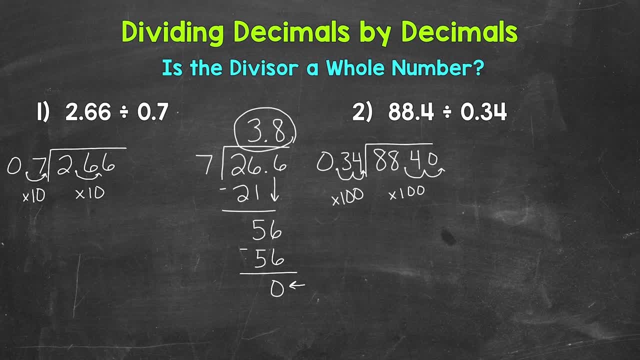 Now we can fill this gap with a zero. Now we can rewrite our equivalent problem with the whole divisor. So we have 8,840 for our dividend and then 34 for our divisor. Now we're ready to go through the division process. Let's start with divide. So we have 8 divided by 34.. How 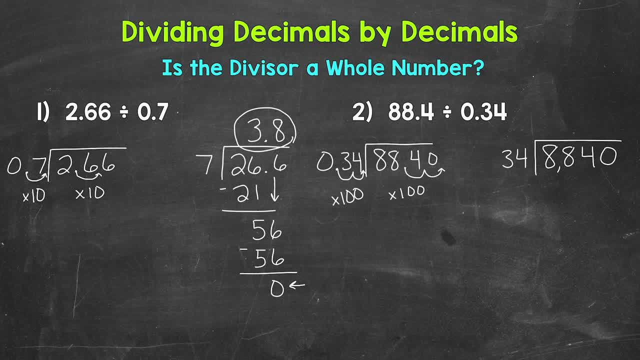 many whole groups of 34 in 8?? Well, we can't do that, So we need to take a look at the next 8 as well and use 88. So we have 88 divided by 34.. How many whole groups of 34 in 88? Well, 2. That gets. 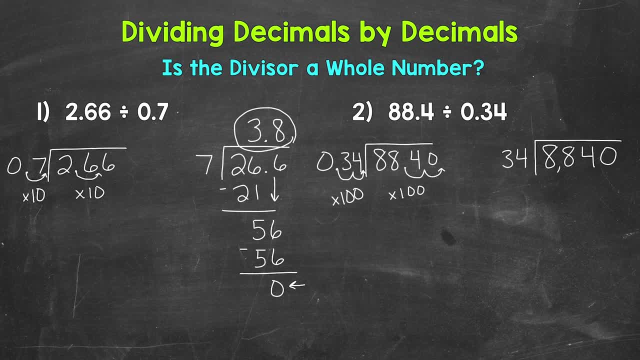 us to 68.. So put the 2 above this 8, not the other 8, because again we used the 88. So the 2 needs to be in the middle. So let's multiply 2 times 34, 68.. Subtract 88 minus 68.. Well, 8 minus 8 is 0. 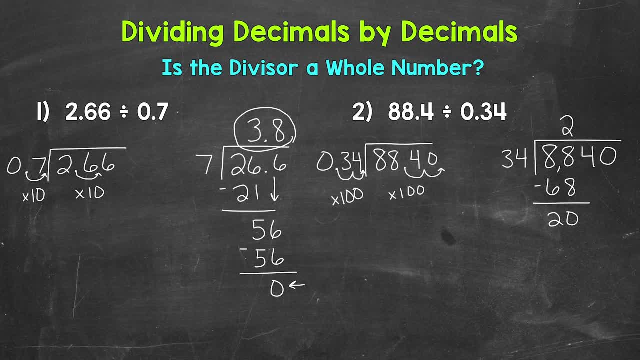 And then 8 minus 6 is 2.. So we get 20.. Bring down And we have 204.. Now we repeat. So we go back to divide. We have 204 divided by 34.. How many whole groups of 34 in 204?? Now for this. 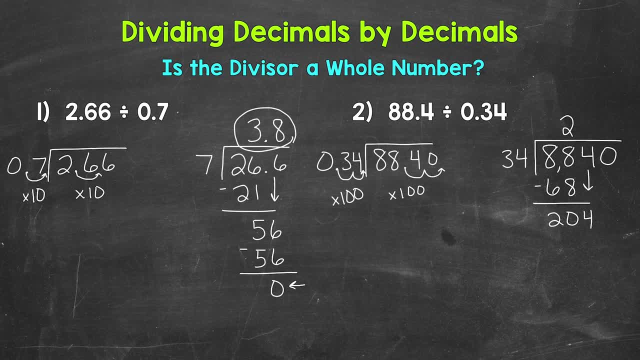 we are going to estimate and check in order to figure out how many whole groups of 34 are in 204.. So let's come to the side here And I'm going to use 34 times 10 as a reference point, So a starting point, Something to go off of 34 times 10. 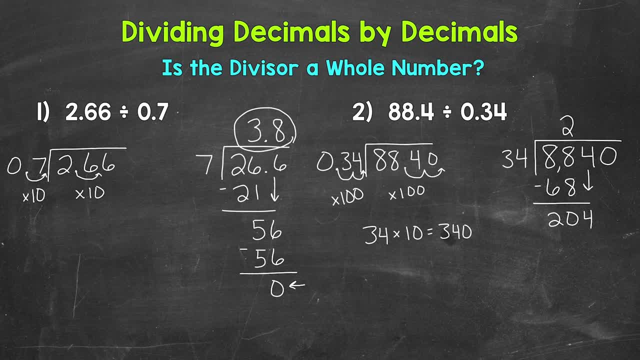 is 340.. Now 204 is quite a bit lower than 340.. So if we know 34 times 10 equals 340, we can base our estimate off of that. So for example, let's try 34 times 7 and see how close to 204 we get. So 34 times 7.. 4 times 7, 28.. 7 times 3 is 21 plus 2, 23.. So 238. 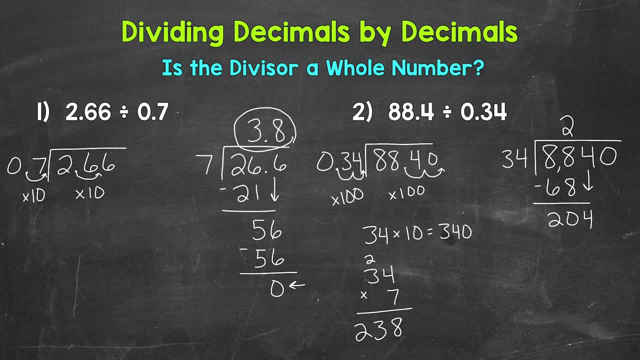 7 was too many, So let's scale that back and try 34 times 6.. 34 times 6.. 6 times 4,: 24.. 6 times 3 is 18 plus 2 is 20.. So we get 204 exactly, So it's going to be 6.. 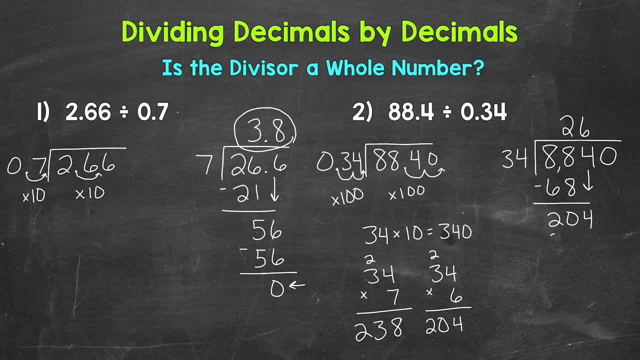 Now we multiply 6 times 34. 204.. Subtract 204 minus 204 is 0.. Now that 0 does not mean we are done. We need to go all the way over within our dividend and bring down all the digits. We still have this: 0. 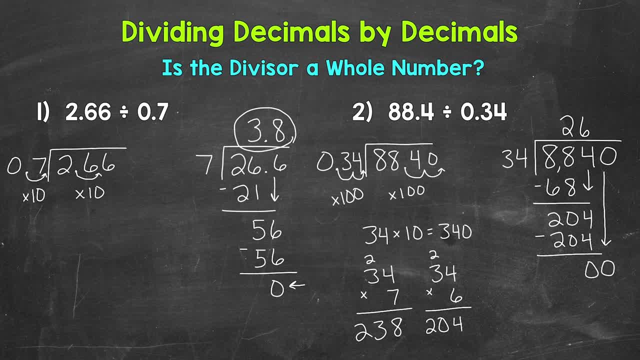 to bring down. So now we have 0 divided by 34. How many whole groups of 34 in 0?? Well, 0.. Multiply 0 times 34. 34. 0. Subtract 0 minus 0 is 0.. Now we went all the way over to the furthest place, to the. 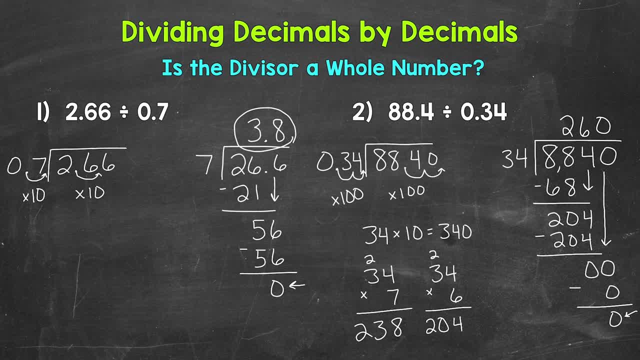 right within our dividend, We have a clean cut: 0.. So we are done. 260 is our final answer for number 2.. So there's how we divide decimals by decimals. Let's move on to dividing by mixed decimals. Here are: 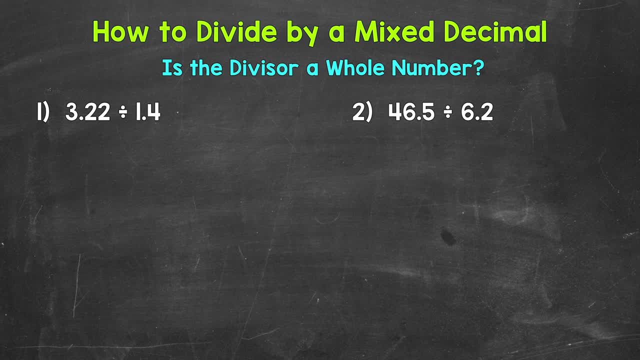 our examples of dividing by mixed decimals. Let's jump into number 1, where we have 3 and 22 hundredths divided by 1 and 4 tenths. Now, the first thing that we need to do, we need to set this problem. 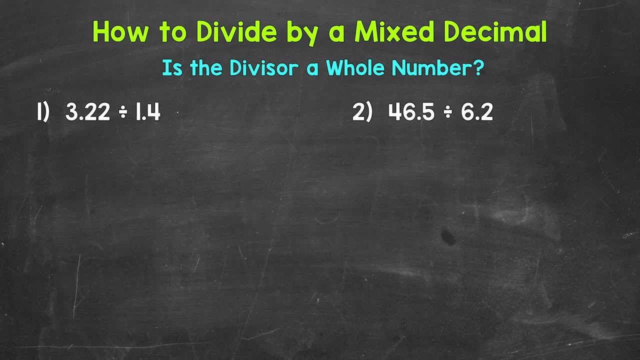 up. That way we can go through the division process. 3 and 22 hundredths is the dividend, the number we are dividing. It goes under the division bar. 1 and 4 tenths is the divisor, the number we are dividing by. It goes on the outside of the 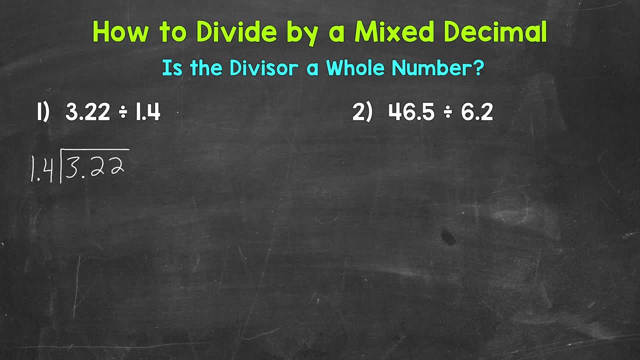 division bar. Now we have our division problem set up, But before we go through the division process we have a division problem that involves decimals. So we always need to check: Is the divisor a whole number? 1 and 4 tenths is not a whole number. That means we need to make it a whole number. 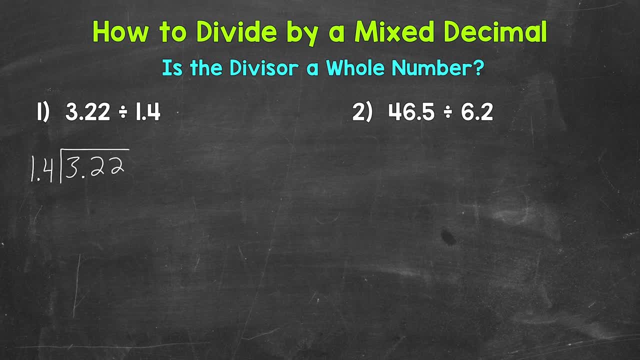 We do this by multiplying the divisor by a power of 10. This will shift the digits to the left and make the divisor whole. Now we can make that very simple and just think of this as moving the decimal to make the divisor whole. For example, let's move this decimal. 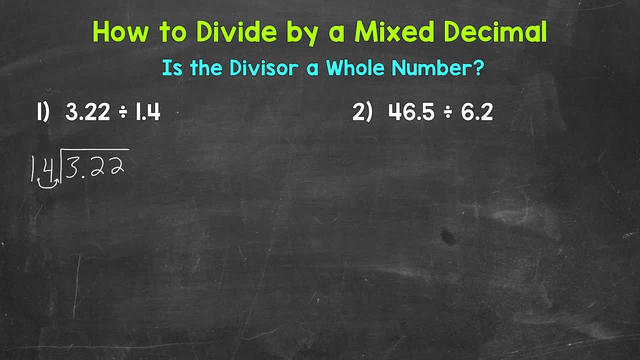 one place to the right, so it goes after the 4 and we have a whole 14.. Now, whatever we do to the outside the divisor, we must do to the inside the dividend. So let's move this decimal once to the right as well. Now again, technically we multiplied the divisor and dividend by a power. 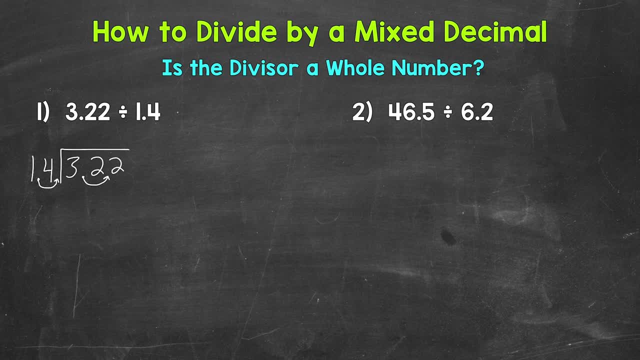 of 10 to shift the digits to the left and make the divisor whole. For example, we multiplied the divisor by 10 for number 1 in order to make it whole. That shifted the divisor to the left and again gave us that whole divisor. We then needed to multiply the dividend by 10 as well. We made 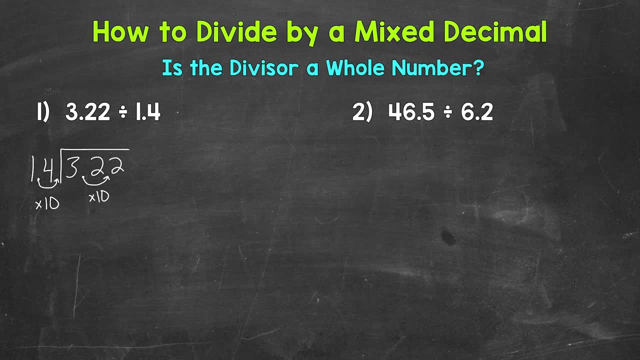 this process simpler to think through by just thinking of this as moving the decimal to make the divisor whole. Whatever we do to the divisor, we must do to the dividend. Making the divisor whole places the decimal for us in our answer and we can make the divisor whole. Now let's 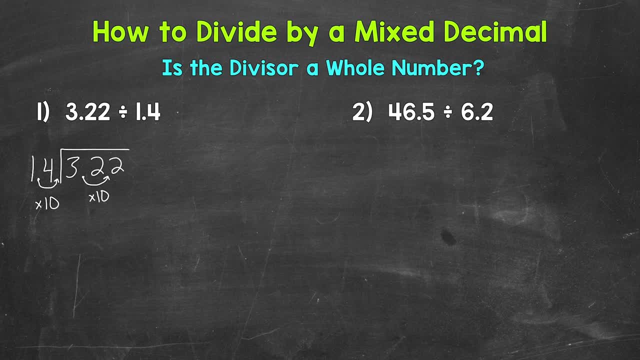 move on to the division process. Since our divisor is now whole, we can go through our division process, The same process we use with whole numbers. So divide, multiply, subtract, bring down, repeat. Now we need to rewrite our new equivalent problem with the whole divisor, So our dividend. 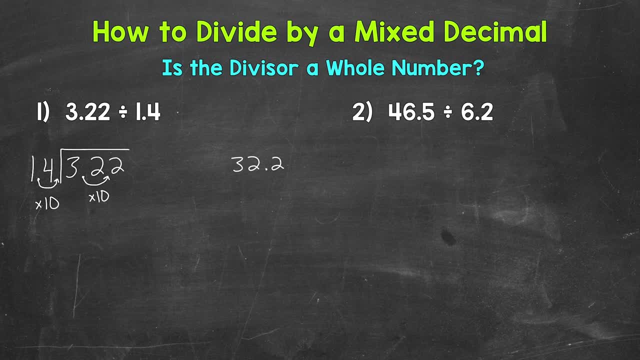 is 32 and two-tenths divided by 14.. Now, as far as our new equivalent problem is the divisor, a whole number. Yes, so we can bring the decimal straight up into our answer. Now let's go through the division process, starting with. 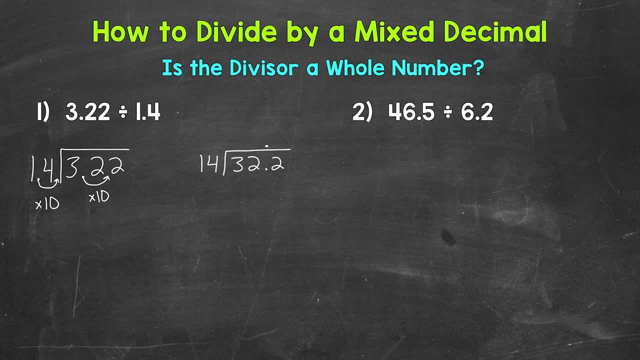 divide. So we have 3 divided by 14.. How many whole groups of 14 in 3?? Well, we can't do that, so we need to use the 2 and look at 32.. How many whole groups of 14 in 32? Well, 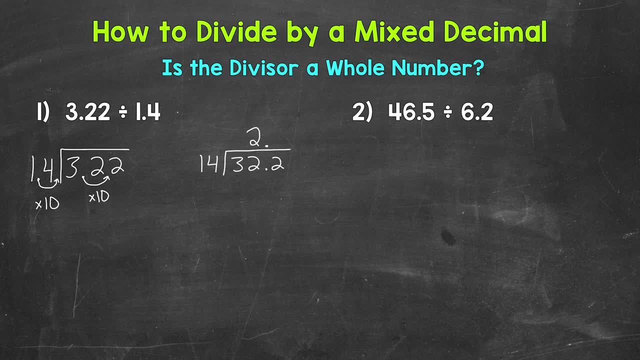 that's 28.. So the 2 needs to go above the 2 in 32, not the 3, since we used both the 3 and the 2.. Now multiply 2 times 14,, 28.. Subtract 2 minus 8, well, we need to borrow. 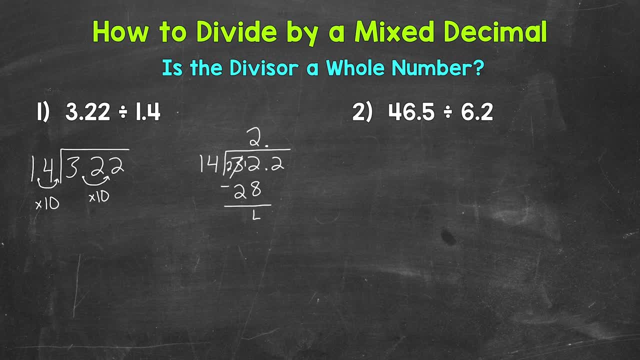 so we have 12 minus 8,, which is 4, and then 2 minus 2 is 0.. So 32 minus 28 equals 4.. Then we bring down that gives us 42, and we repeat. so we go back to divide. 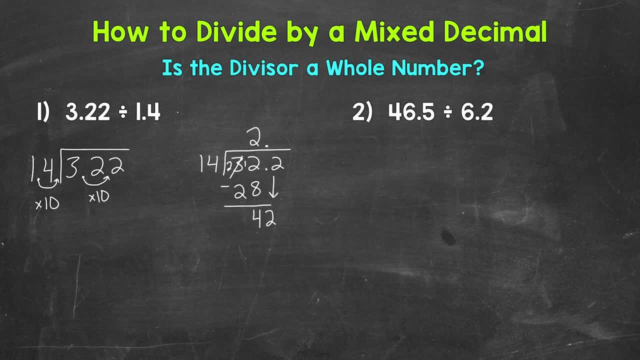 We have 42 divided by 14. How many whole groups of 14 in 42?? Well, 3.. That hits 42 exactly. Multiply 3 times 14, 42, subtract 42 minus 42 is 0.. 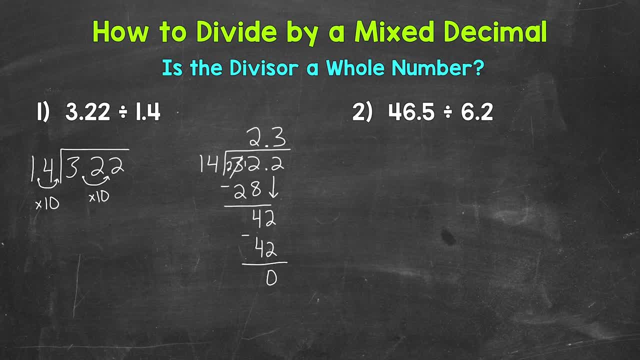 We went all the way over to the right within our dividend as far as bringing digits down, and we have a clean-cut 0 at the end. so we are done Our final answer: 2 and 3 tenths. Let's move on to number 2, where we have 46 and 5 tenths divided by 6 and 2 tenths. 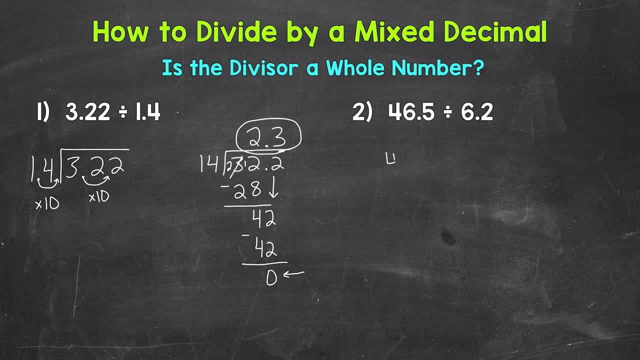 Let's set this problem up: 46 and 5 tenths. 5 tenths is the dividend, the number we are dividing 6 and 2 tenths is the divisor, the number we are dividing. by Now that we are set up, we need to check: is the divisor a whole number? 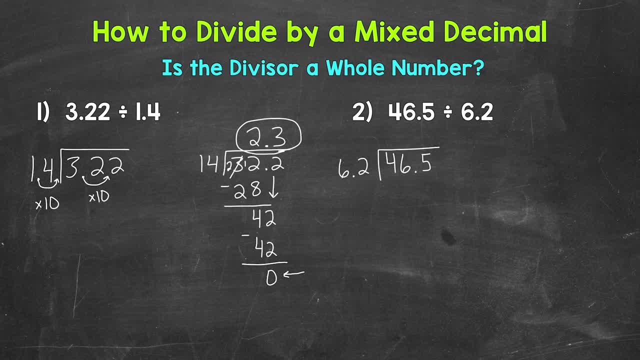 6 and 2 tenths is not a whole number, so let's make it a whole number. Let's move the decimal once to the right, So now we have a whole 62.. Technically, we multiply, Multiplied our divisor by 10.. 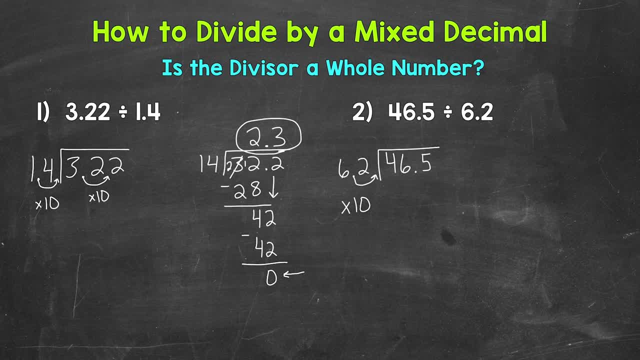 That was the power of 10. we multiplied the divisor by Now. whatever we do to the outside the divisor, we must do to the inside, the dividend. So let's move this decimal once to the right as well, And again, technically, we are multiplying our divisor and dividend by 10.. 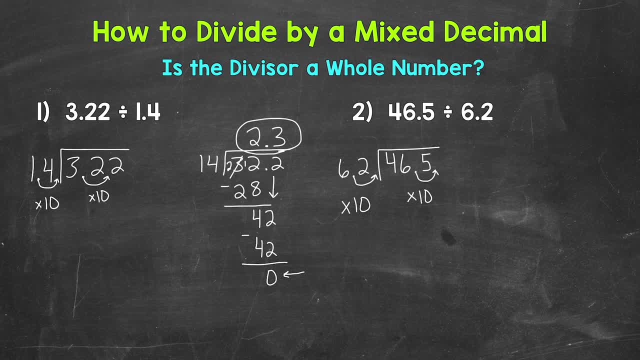 Now we have a whole divisor so we can rewrite our equivalent problem. We have 46.. 65 divided by 62. Now that we have our rewritten equivalent problem with a whole divisor, we can go through the division process, starting with divide. 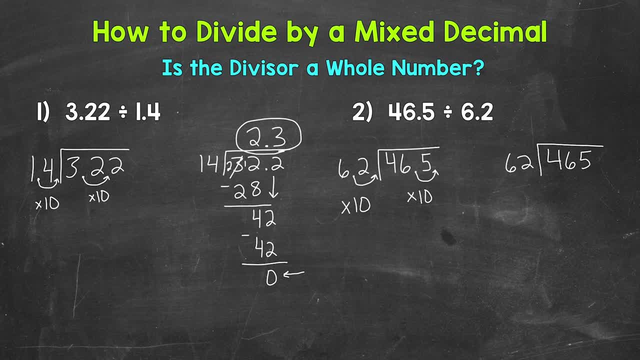 So we have 4 divided by 62. How many whole groups of 62 in 4?? Well, we can't do that, so we need to use the 6 and take a look at 46.. How many whole groups of 62 in 46?? 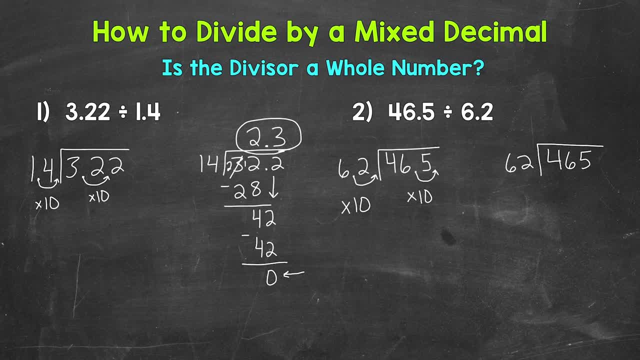 Well, we can't do that either, so we need to use the 5 and take a look at 465.. How many whole groups of 62 in 465?? We're going to need to estimate and check in order to figure this out. 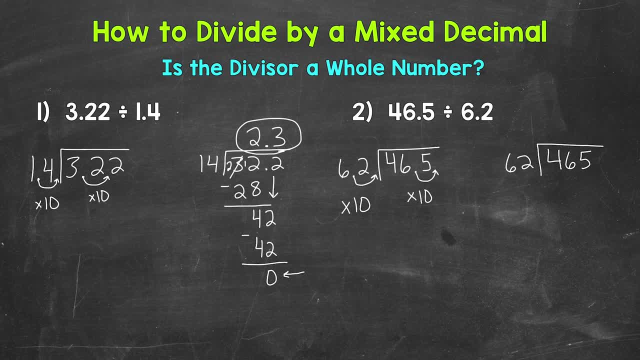 because I don't know how many whole groups of 62 are in 465.. So let's come to the side and again estimate and check. I'll use 62 times 10.. As a reference, a starting point. we know 62 times 10 is 620.. 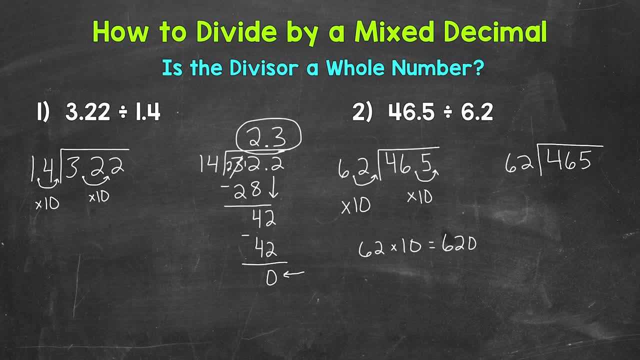 That gives us something to go off of. We can base our first estimate off of 620 and go from there. 465 is less than 620, but it's kind of close. so let's back up from 10 and try 62 times 8 and see how close we get. 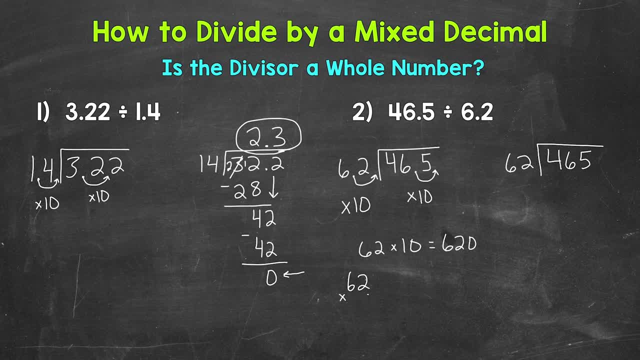 So let's multiply. Let's multiply 62 times 8 and again see how close we get. We are estimating and checking 8 times 2, 16.. 8 times 6, 48.. Plus 1, 49.. 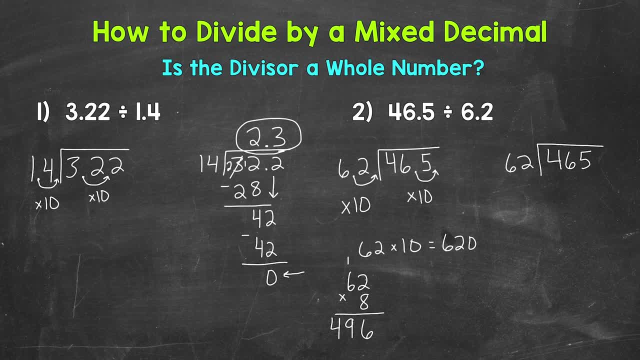 So we get 496,, which is too much, So we need to back it up. Let's try 7.. 62 times 7.. 7 times 2, 14.. 7 times 6, 42.. Plus 1, 43.. 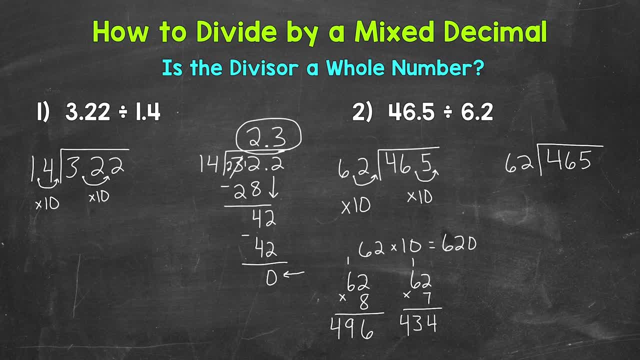 So 434.. It's going to be 7 whole groups of 62. So put the 7 above the 5, since we used 465.. Now multiply 7 times 62, 434.. 7 times 6, 434.. 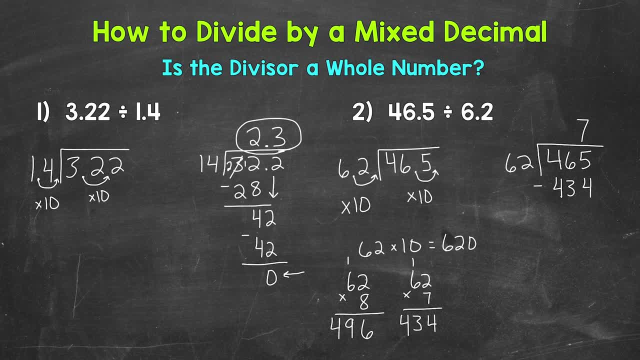 7 times 6, 434.. Subtract: 5 minus 4 is 1.. 6 minus 3 is 3.. 4 minus 4 is 0.. So we get 31.. So 465 minus 434 equals 31.. 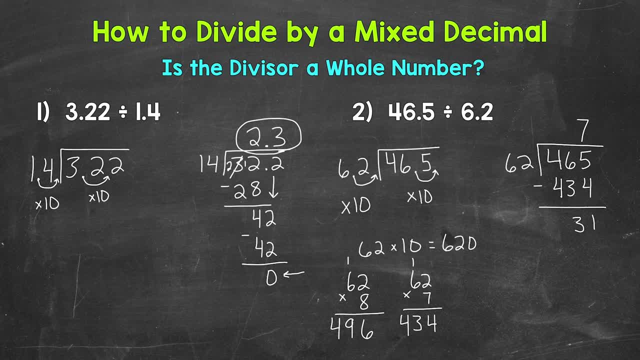 Now we are at the bring down step, But there's nothing else to bring down And we don't want to write 7 remainder 31.. We are working with decimals, so we want to keep everything in decimal order, decimal form, even the answer. So we need to continue this problem. So what we can do, we can. 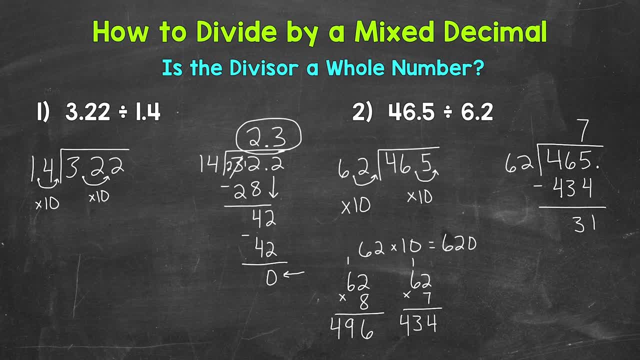 place the decimal in our dividend. A decimal comes after a whole number, so after 465.. Then we can write a zero in the tenths place. Now we're able to bring that zero down and continue the problem. That zero to the right of a decimal does not change the value of the problem We still have.